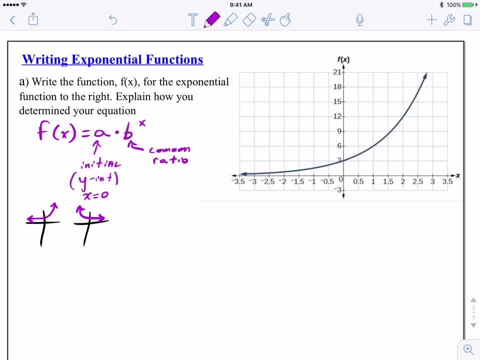 the y-axis. So what's the difference between these? It all relates to the base b, what we said, the pattern, what you're multiplying by: If b is anything greater than one, it will be an increasing function. If b is anything less than one, it will be a decreasing. 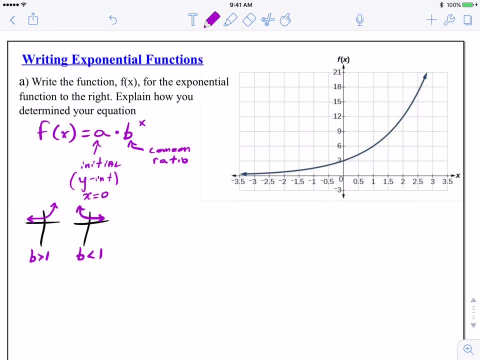 function be getting smaller and smaller. This has to do with basic exponent concepts. If you have something like one half and you're raising it to a higher power, it's going to get smaller. You'll have like one half, one fourth if you're raising it to the second power. let's say 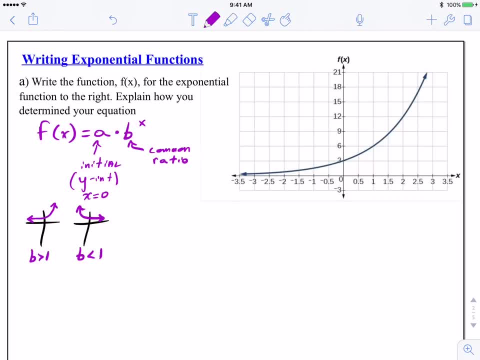 Whereas with anything bigger than one, obviously it gets larger as we make that a bigger exponent. So we want to keep that in mind And just by looking, we should note that rb is probably going to be the left case here, Since we have an increasing function. That's obviously useful to know If you write the 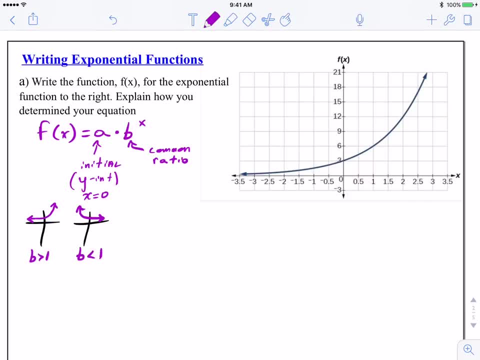 equation rule and then you realize like, oh man, I have a fraction in there. and you look at your graph and you see an increasing function. obviously something's off And it doesn't hurt to know it either. So let's start. When you're doing these, 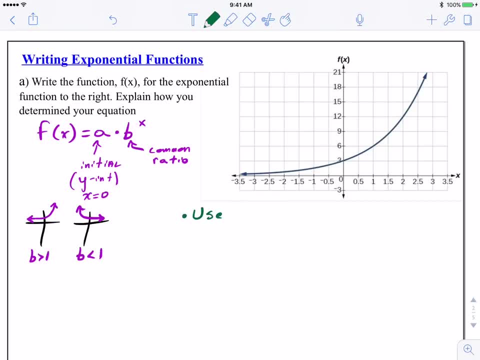 some things that I would make a note of. you want to use nice or good points, if you want to call them that. It's not a technical term, so I'm putting it. I'm putting it in parentheses. What do I mean by nice points? 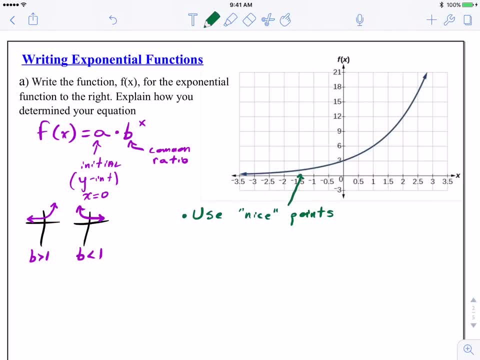 I'll give you an example of what they're not. This would not be a nice point right here, Right, I'd be guessing if, at whatever the y value is there, I have no idea what that is. Maybe it's a half, maybe it's a quarter. Nice points are points that actually hit. 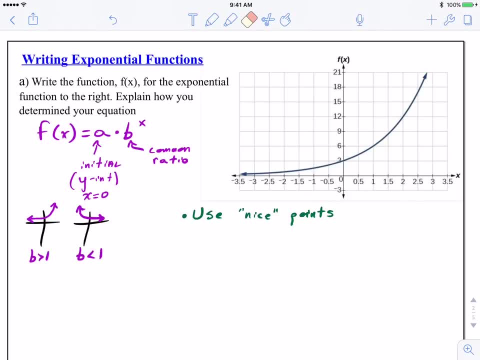 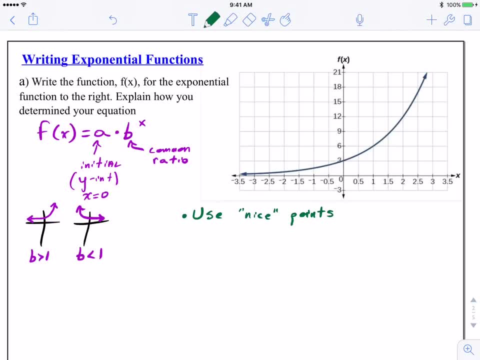 This is where it is. I'm not guessing. So some nice points that I see. luckily, the y-axis is nice. This point looks pretty good. This one is a few nice ones. It's a pretty nice graph we have here. So now that we have those few points, 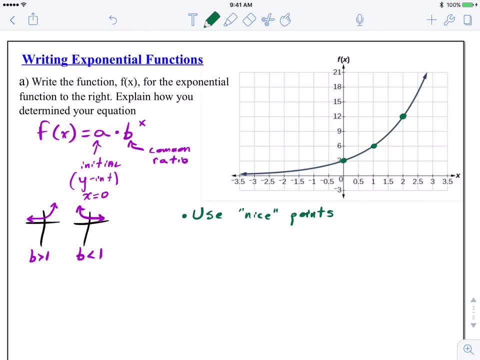 those few nice points identified. we're going to try to look for a pattern, something we notice that's happening, maybe One thing we got lucky with here, and we're going to take a look at another example in a second where we don't see this. 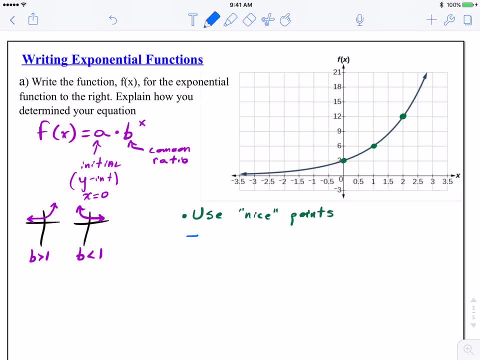 luckily the y-intercept was one of those nice points, So right away I know the a value or the y-intercept, which is three, And that was right here. It clearly passed through three. Sometimes they make these harder by making them not pass through that point. So we'll take a look at what happens when we see something like. 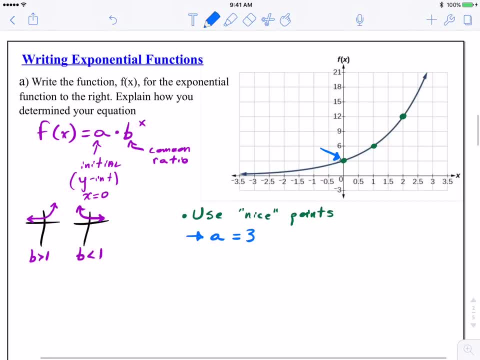 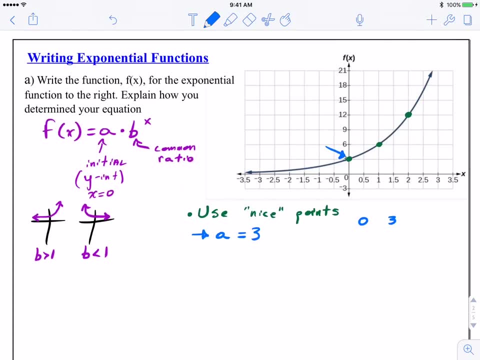 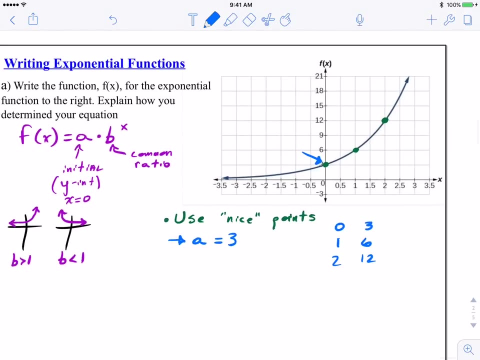 that in a second. Now the pattern here I notice. I'm going to write them down, just so we can see it a little bit. a little bit differently: When x is zero, we have three, When x is one, we have six, And when x is two, we have 12.. I'm just writing down the coordinates. 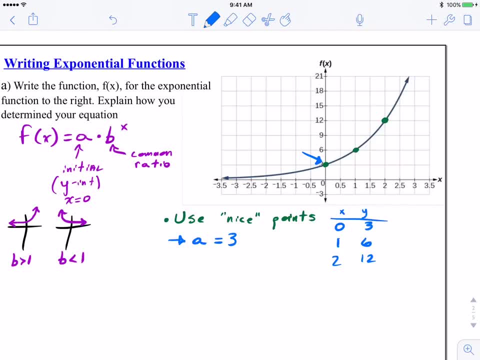 almost like a little table, Okay. so what's the pattern? Now that we see it this way, it's pretty clear that in each case we're doubling. Okay, we're going times two each time, So this would make our b value our base. 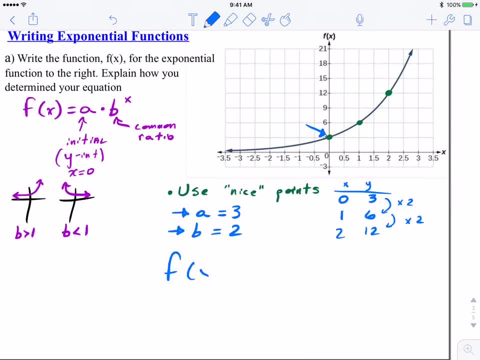 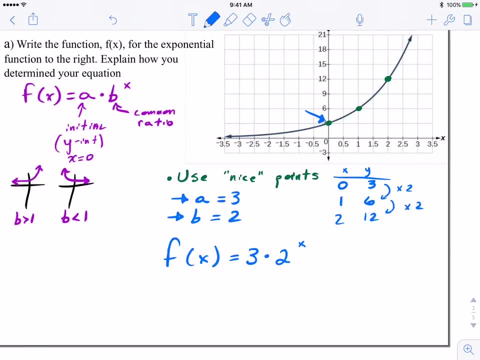 two. Now I have everything I need to write the actual function rule. so I'm going to do that. So I'm going to do this. Remember: one thing you do not want to do is this: That would be a huge mistake, a huge conceptual error. that, hey, I can multiply things that have. 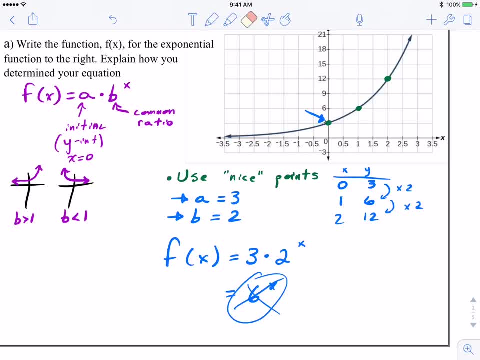 exponents attached to them. Obviously, we cannot do that. I don't even want to leave it on the page, just to confuse anyone. So that would be your final answer, Putting the two in parentheses. if that helps you separate it, that's fine. 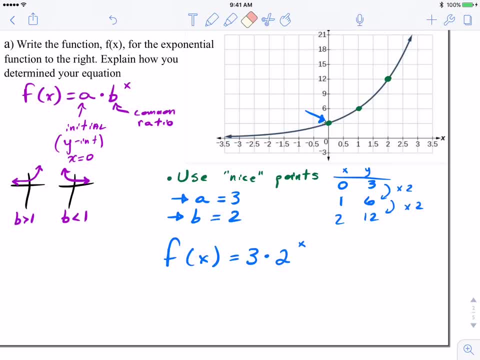 But three times two to the x power. Another option: I unfortunately don't have my calculator- a graphing calculator- on my iPad, but on your TI-84, I'll write down the buttons. you can hit stat. So this is a different strategy that I mentioned earlier. You would hit stat, select. edit. 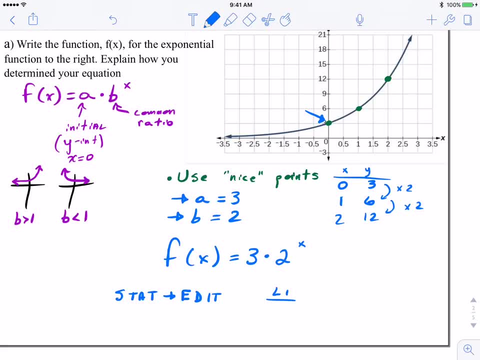 And under list one, you would type in the x values of those points. Under list two, you would type in the y values of those nice points. You actually only need two of them. So you could do something like this: You could do zero, one and three, six, Typing in: 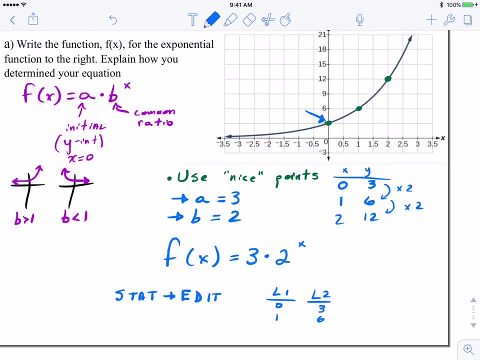 the third one won't hurt, but it's just not needed. So you would type those in, Then you would hit stat calc. So hit the stat button again. but now you're going onto calc. Make sure that these correspond as well. And you're going to select zero. Just hit the zero button. 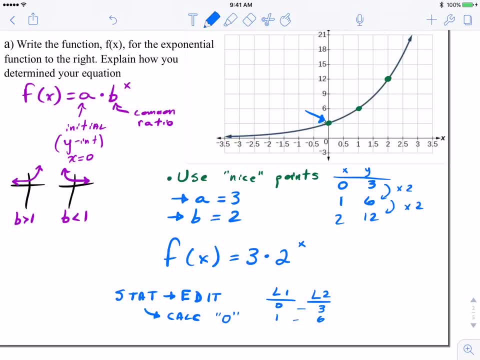 or you could scroll down. It'll say expreg, which is exponential regression, And it will literally spit out that same formula for you. It even gives you the format up here, the a times b to the x, to remind you what it should look like. So that's a calculator option. 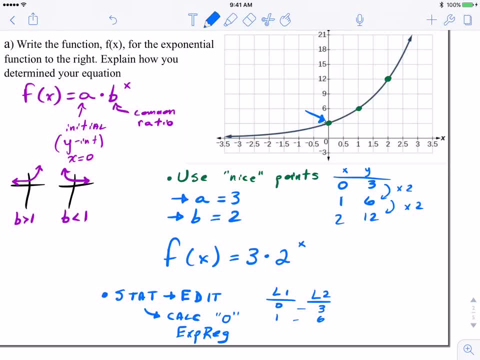 And obviously all the work we've shown here. and even if you did the calculator strategy, this would be our explanation. We don't have to write a formal essay on what we've done, but we could just say something along the lines of: 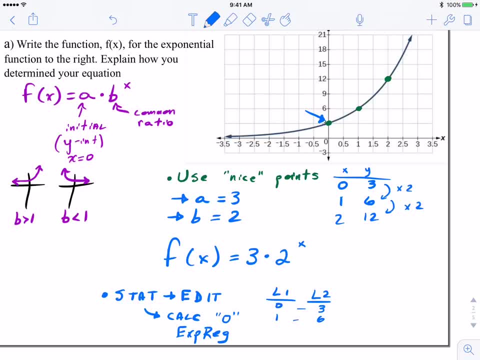 I used the table feature on my graphing calculator and I did an exponential regression and this is the equation I got, Or the algebraic approach, we could say: I found the y-intercept and I found the common base, the common ratio, to be two. 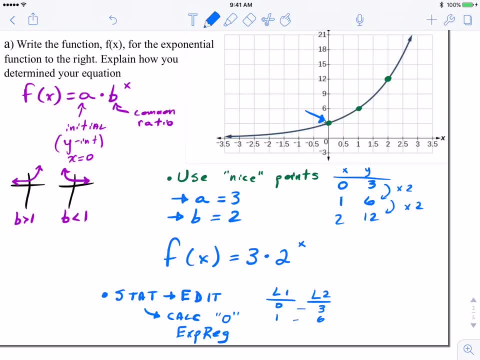 And all of our work is justifying that. So we've explained kind of how we came up with it. I also made note I did call it f of x. That's something we want to focus on: using proper terminology, not to lose a silly half a point or a point along some way. 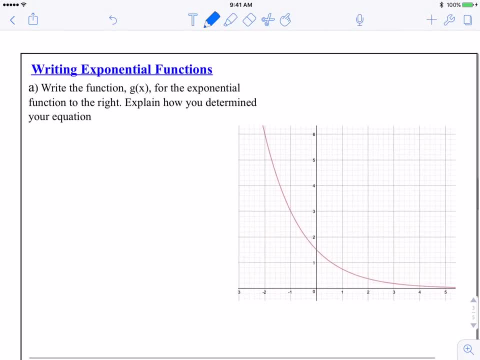 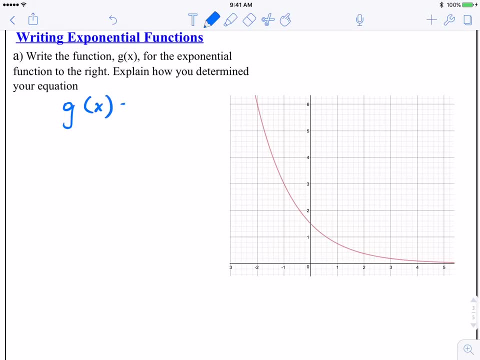 Okay, so quickly, let's take a look at that other case, And you see what I'm. in this case we're looking at g of x, So I'm going to write down that same definition. This is what I was mentioning earlier. Now we don't have a y-intercept. 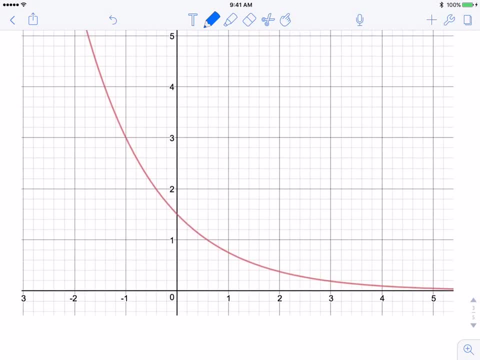 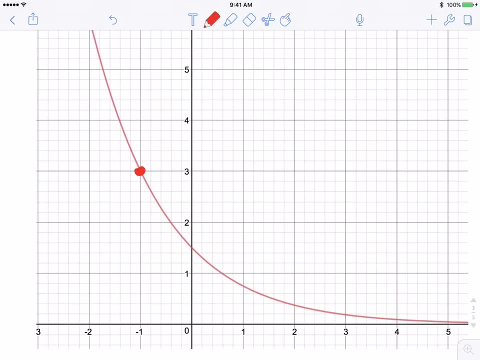 Okay, there is a y-intercept physically, but we don't have one that I could clearly see. It's not a quote-unquote nice point. So I'm going to highlight the nice points. I think I only actually see two of them. Okay, two nice points over there. 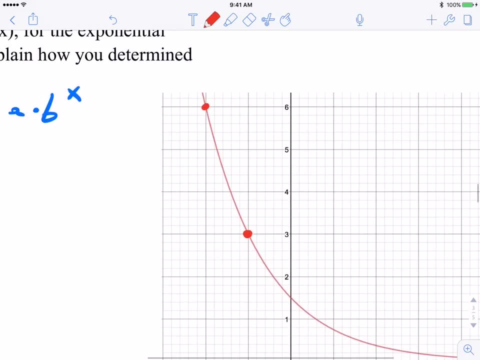 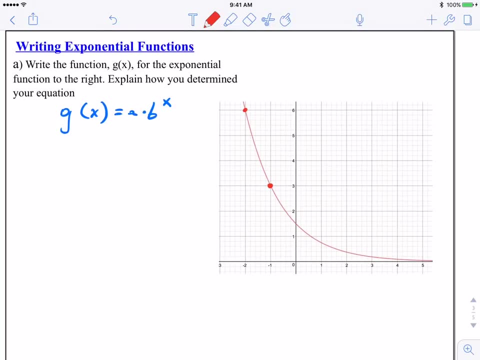 and everything's fractional on the other side. Nothing even that I could make like a quarter or half or something like that. So not a problem. Exponential functions are actually defined by just two points, So I'm going to write them down. we have negative 2, 6. And negative 1, 3.. 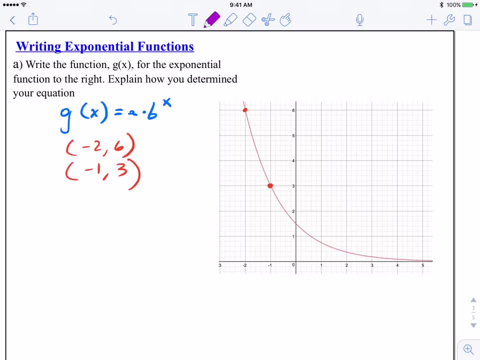 Okay, So in this case we don't have this to be a definition, but we do have a independent function which we basically call But unknown. So in this case we don't have a a y-intercept, That would be where x equals 0.. So I can add that We can pick out a pattern. 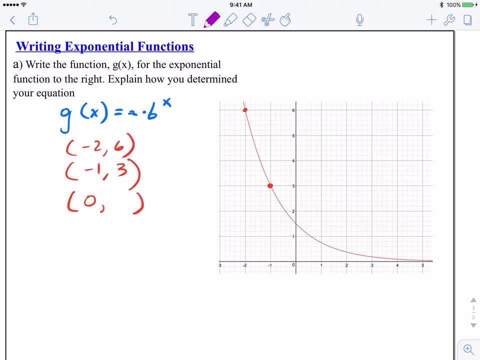 Luckily these are right next to each other: negative 2 and negative 1.. So I'm not skipping anything. There's no jumps, like we say. I can just strictly say: hey, what did I have to do to go from 6 to 3?? In this case, we always want to think in terms of multiplication. You don't? 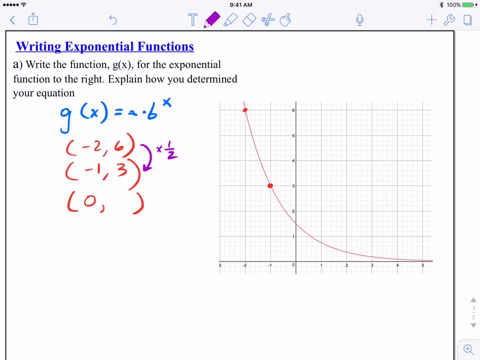 want to say division. This would be multiplying by a half, So I already found b relatively easily, Um. now I'm going to continue this one step further. You might say what's the point of that Um? by having a point that starts with 0. 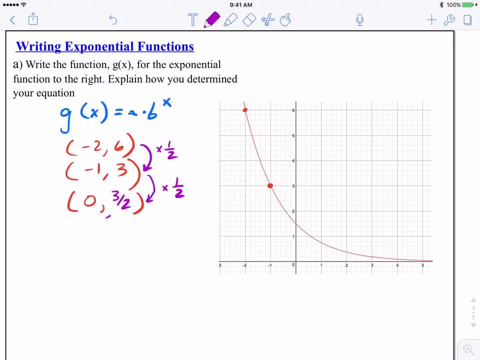 and having the y-value that goes with it. what did I just find? What does this point represent? This is the y-intercept. Okay, You can do it in this coordinate way. You could write it however you want. You can make a table and do this pattern. 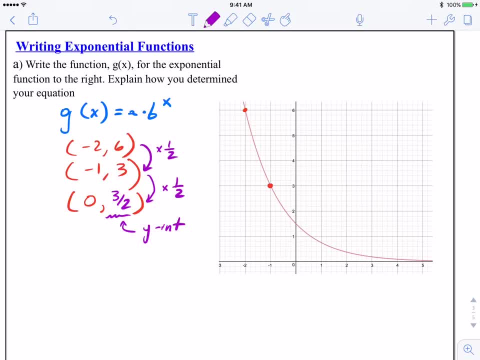 Whatever works for you, But I've just found the two things that I need here. I found the common base, the pattern times one half Um, and I found the starting value, the y-intercept, or where x equals 0.. Sometimes this might be off. 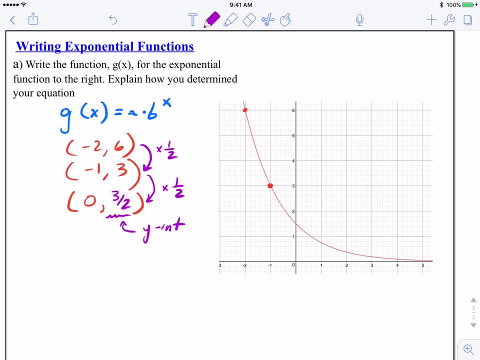 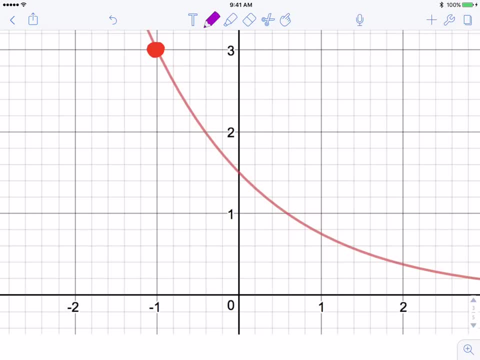 a little bit. Maybe we have to go two or three jumps, But in this case we just had to do one. It also kind of makes sense. Three and a half is 1.5. And if we look closely it looks right around. 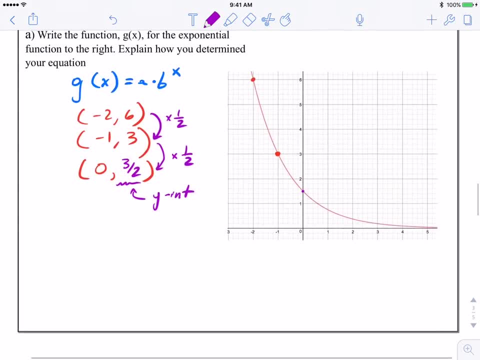 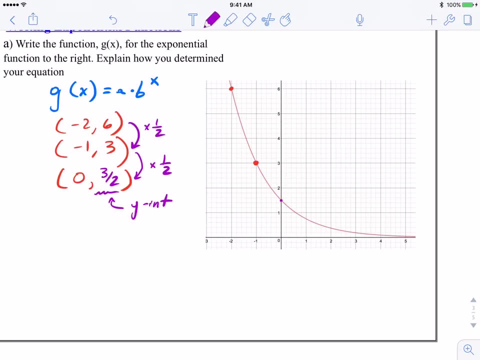 kind of makes sense. Um, I wouldn't want to say that just by looking at the graph, but now that we see it's actually 1.5, it does make logical sense. Also what we mentioned earlier, once we put our function together. 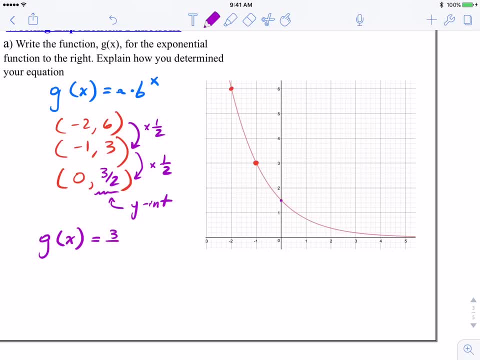 here. let's look at the base that we get. So 3 over 2 or 1.5 works And the common multiplier is one half to the x power Um we mentioned earlier. if the base is less than 1, it should be a. 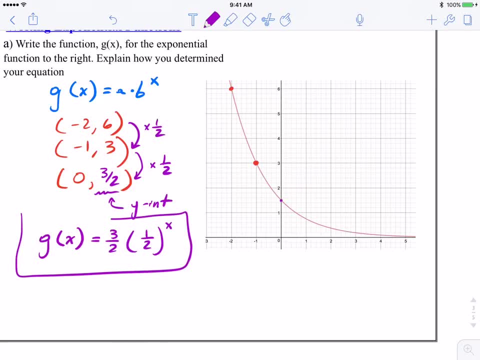 decreasing function, which this is: Everything works out, Everything passes. all our little mental tests that we, you know, check everything with Um and that's g of x. So this is writing the equation of an exponential function. Hopefully this helped. Thanks for watching.